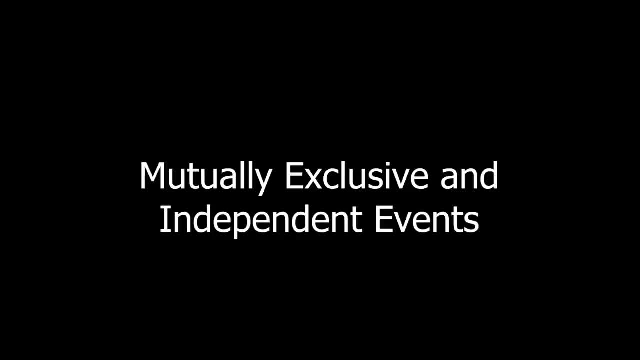 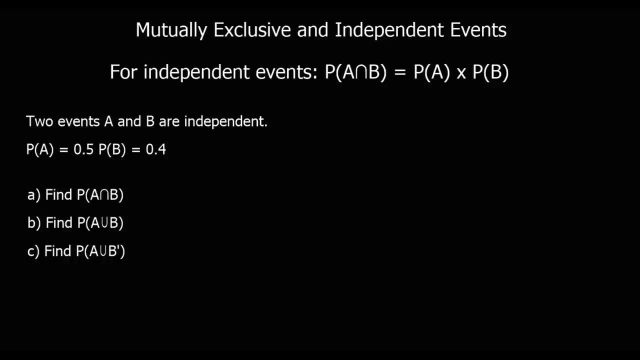 In this video we're going to look at mutually exclusive and independent events. We're going to start with independent events. So for an independent event, the probability of A and B is equal to the probability of A multiplied by the probability of B. So if A happening, 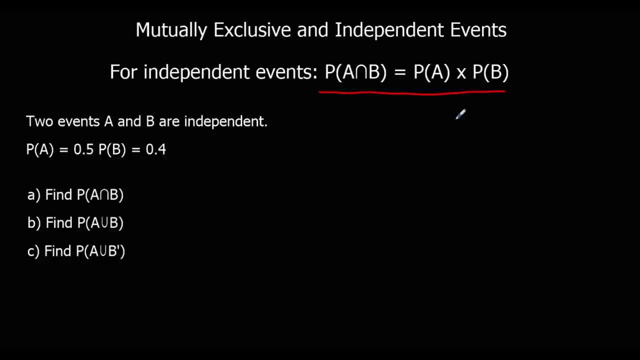 doesn't affect B. so if A happening doesn't affect the probability of B happening, then the probability of both of them happening together is simply probability of A multiplied by the probability of B. So in the question here we're told two events are independent and the probability of A is 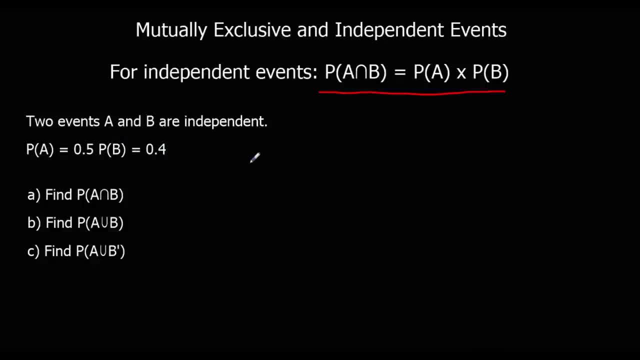 0.5 and the probability of B is 0.4.. So that means the probability of A and B is 0.5 times 0.4 and that's 0.2.. So now we can draw a Venn diagram for this information. 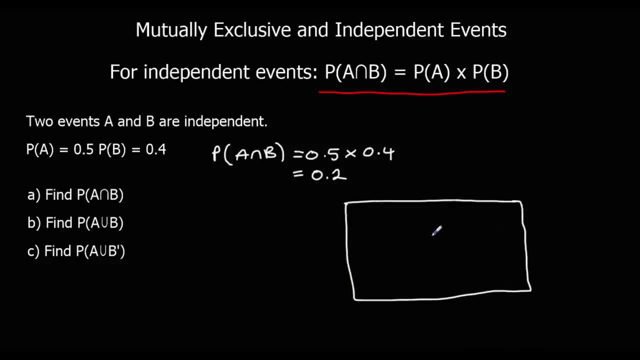 So we've got A and B. Our middle bit is 0.2.. The probability of A is 0.5.. We've already got 0.2.. So we need another 0.3.. The probability of B is 0.4.. We've already got 0.2.. So we 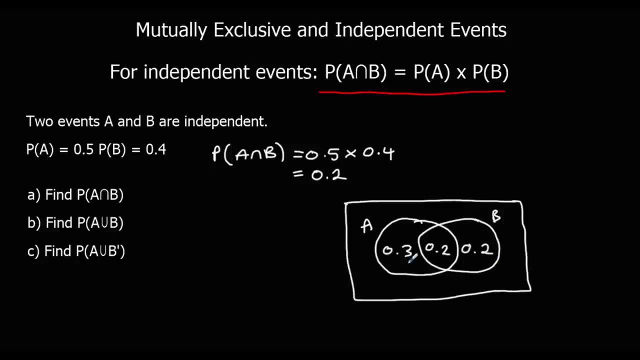 need another 0.2. And here we've got 0.7.. So we've already got 0.2.. And here we've got 0.7.. So we need another 0.3.. The probability of A and B to answer the questions now, that's. 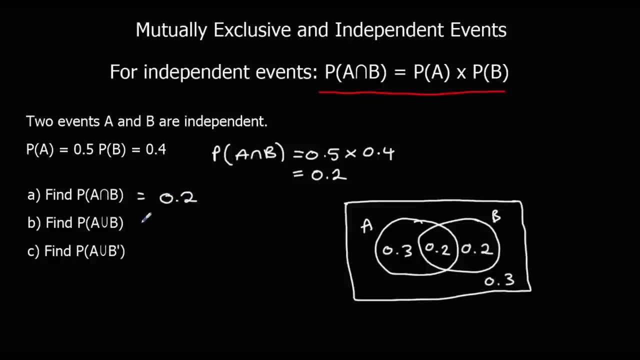 0.2.. We've already worked that out. The probability of the union of A and B, that's all the circles together. So 0.3 plus 0.2 plus 0.2, that's 0.7.. 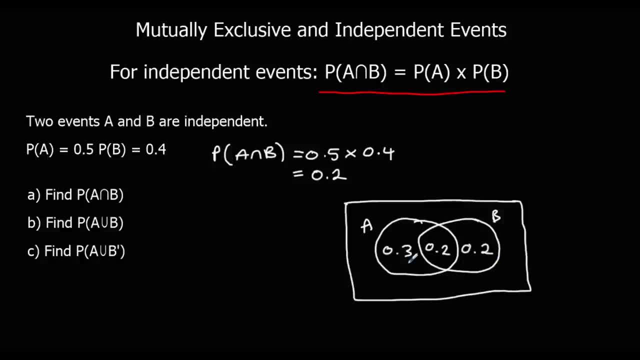 need another 0.2. And here we've got 0.7.. So we've already got 0.2.. And here we've got 0.7.. So we need another 0.3.. The probability of A and B to answer the questions now, that's. 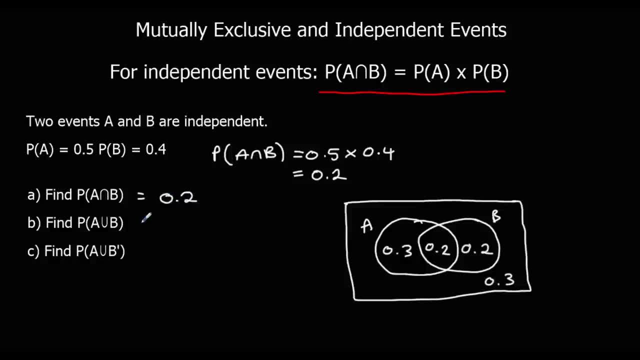 0.2.. We've already worked that out. The probability of the union of A and B, that's all the circles together. So 0.3 plus 0.2 plus 0.2, that's 0.7.. And the 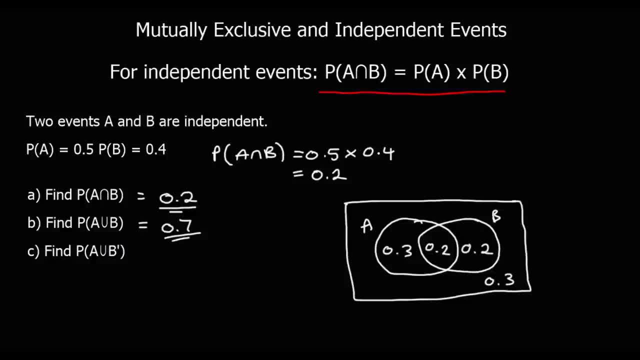 probability of B. a and B and together minus 0.2, plus 0.7 divided by B times 0.2, so we need of A, the union of A and not B. so these two bits are A, not B. is these two bits? 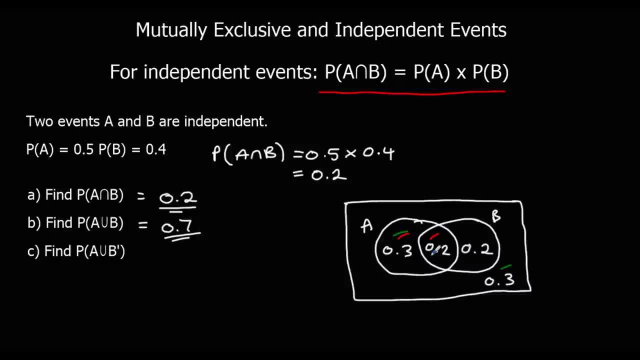 and it's a union. so we want all of that together, which is 0.3, 0.5, 0.8. okay, here's another question. you could pause the video and try this one, okay, so again we've got independent events. so that means the probability of A and B is just the two probabilities multiplied together. 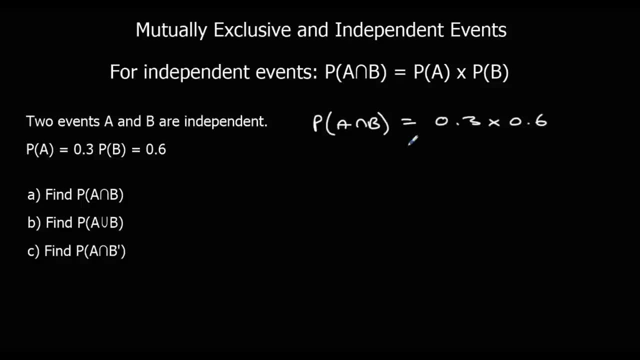 so 0.3 times 0.6, that's 0.18, and we can draw a Venn diagram. we've got A and B, 0.18 in the middle. the probability of A is 0.3, so we need another 0.12. 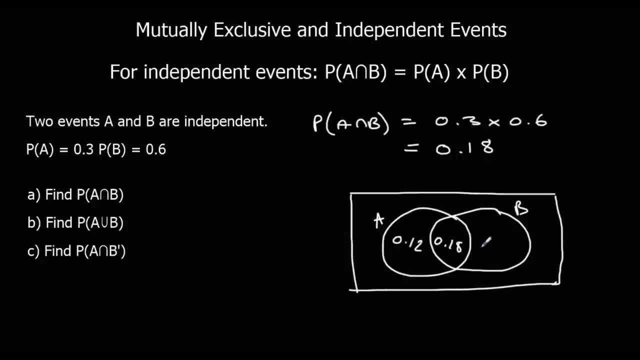 the probability of B is 0.6, so we need another 0.42 and we've got B is 0.6 plus 0.12- 0.72, which means we've got 0.28 left. so okay, the questions for the probability of A and B: we've worked out 0.18. 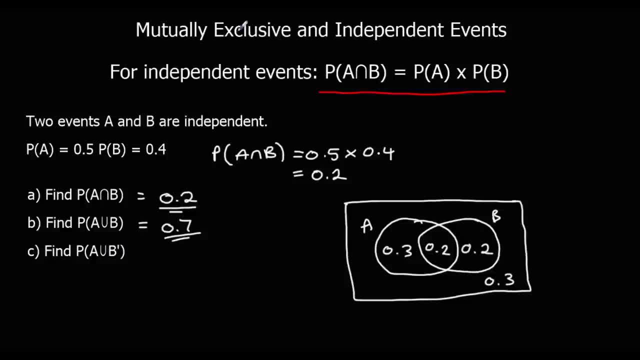 And the probability of the size monitors both here and above. so they both normally of A, the union of A and not B. so these two bits are A not B, is these two bits and it's a union. so we want all of that together, which is 0.3, 0.5, 0.8. okay, here's. 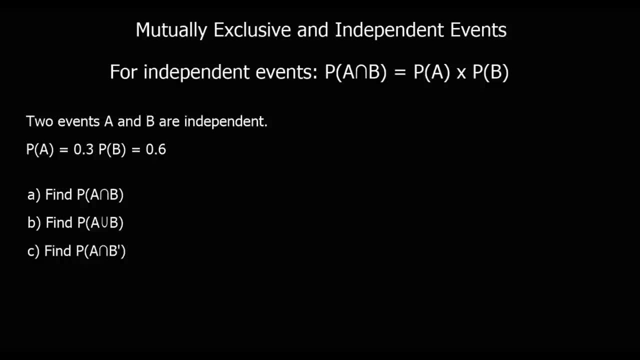 another question. you could pause the video and try this one. okay, so again we've got independent events. so that means the probability of A and B is just the two probabilities multiplied together. so 0.3 times 0.6 that's 0.18 and we can draw a Venn diagram. 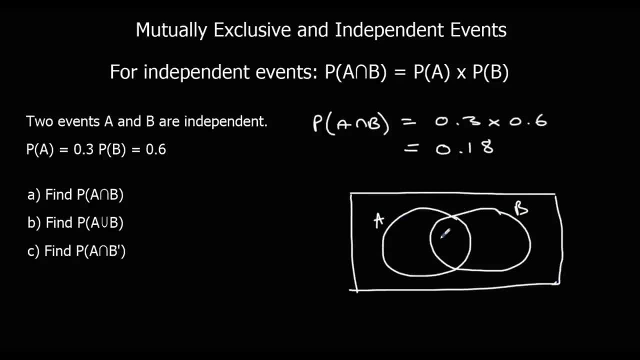 we've got A and B 0.18 in the middle. the probability of A is 0.3, so we need another 0.12. the probability of B is 0.6, so we need another 0.42 and we've got B is 0.6 plus 0.12- 0.72. 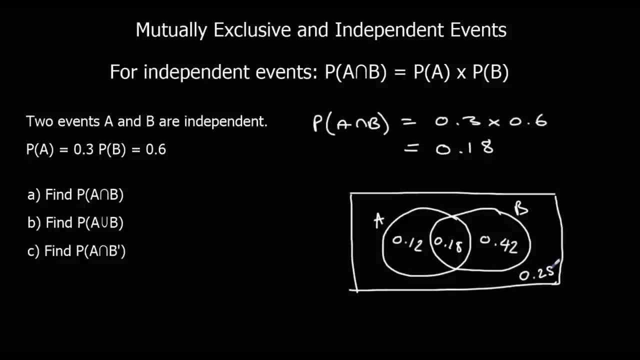 which means we've got 0.28 left. so okay, the questions. for the probability of A and B, we've worked out 0.18, the probability of the union of A and B. so that was all the circles together, that was 0.72. 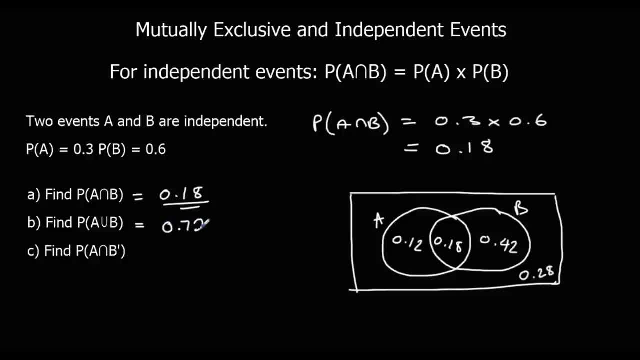 and the probability of A and not B. so these two bits are A and B. oh wait, a second. and the probability of A and B. so this means both of them. and these two bits are instead of B and means both of them. so which bit's got both the lines? there's 0.12. 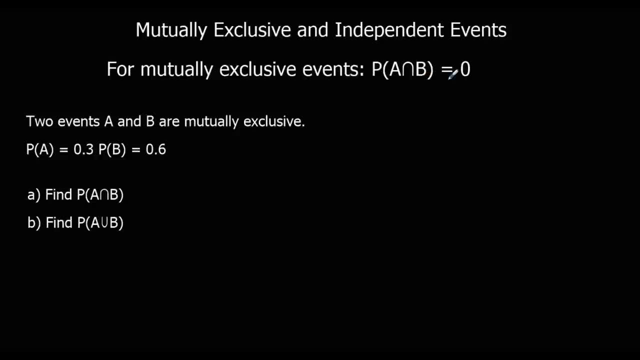 okay, mutually exclusive events. so mutually exclusive events cannot happen at the same time. so A and B is 0 and B and it can't happen at the same time. 1. there's only 1, 0, 0, risks and this is the essential up, left and right, left part of the pair, of the pair, but B or A and B, 2.0. And so what about the cross section? 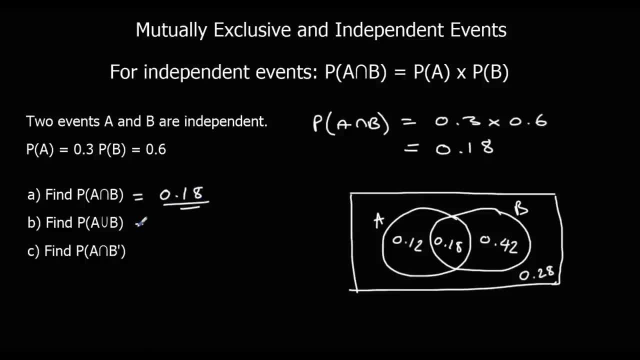 the probability of the union of A and B. so that was all the circles together. that was 0.72 and the probability of A and not B. so these two bits are A and B. these two bits are not B and means both of them. so which bit's got? 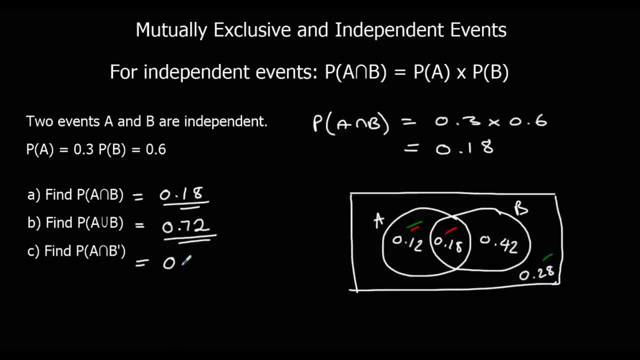 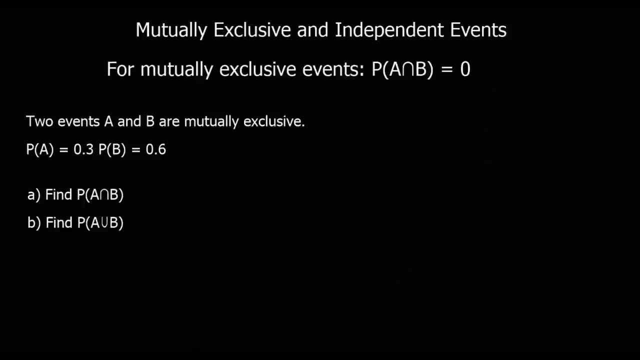 both the lines, the 0.12. okay, mutually exclusive events. so mutually exclusive events cannot happen at the same time. so a and B is 0 and B is 0. yeah, these two things are the dots. so, Okay, mutually exclusive events cannot happen at the same time. so they are the. 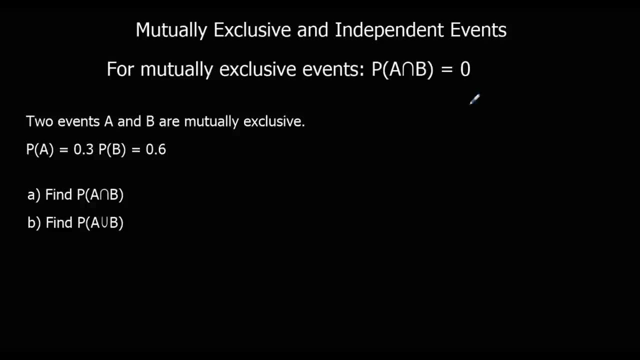 they can't happen at the same time. so the chance of them both happening at the same time is zero. so if we've got probability of a is 0.3, probability of B is 0.6. the Venn diagram for mutually exclusive events actually looks like. 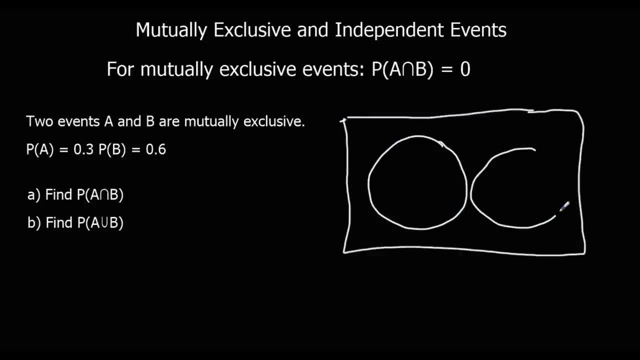 this, so there's no need to have an overlap because there is no chance of them happening at the same time. so we've got 0.3 0.6. so the outside is 0.1. so the probability of A and B: well, they can't happen at the same time, so it's. 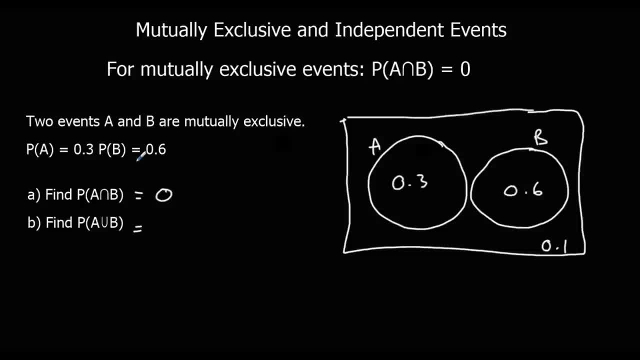 zero. and the union? well, it's just the two added up, so 0.9, okay. another question on mutually exclusive. give this one a go quickly, okay. so mutually exclusive events, A and B- zero chance of happening. the union of A and B is just the probability of A plus the probability of B, so 0.7. 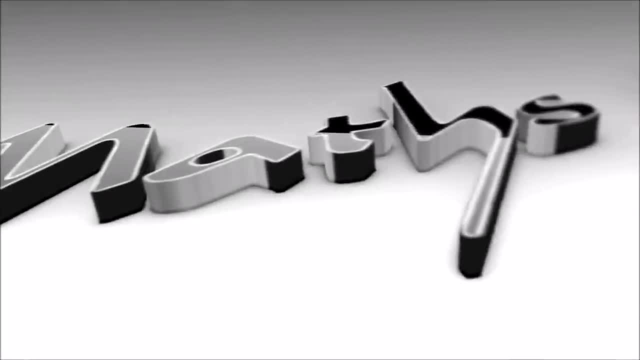 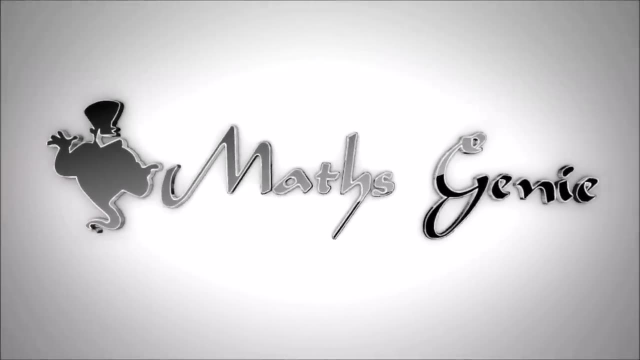 is zero and the union of A and B is 0.7, so it's just the probability of one partner being the union of all. partners are very close, so this is a very interesting subject and that's a really interesting question. it's not a very specific question, but it's a very original question but you're probably all kind of familiar with this. you might make the same question, but it's still the same question and it's very interesting. so at least it is the same thing and it's really interesting to me.